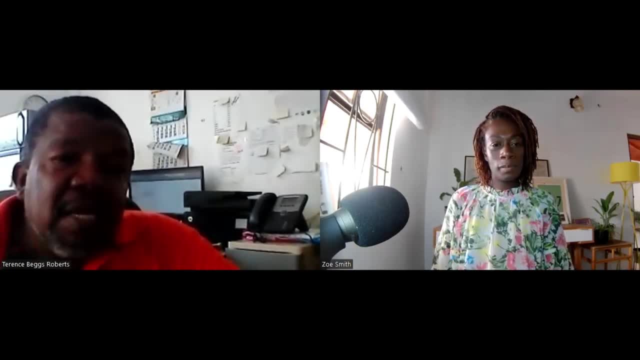 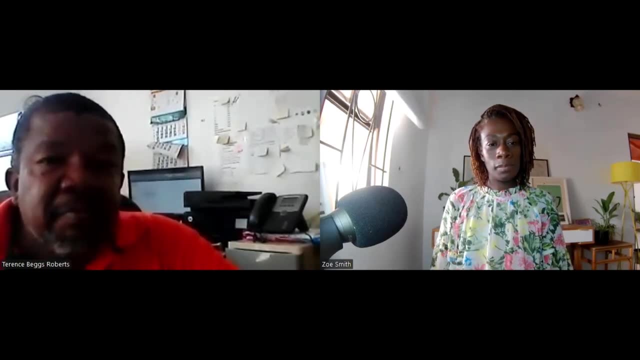 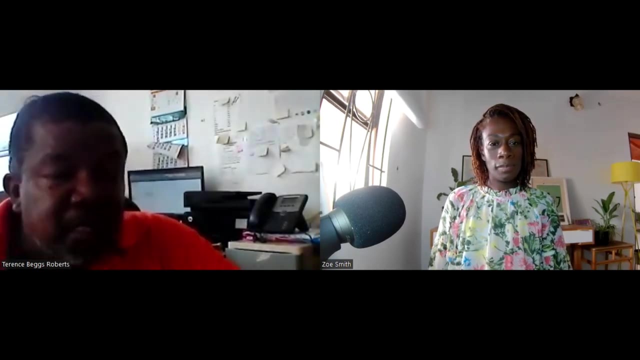 finds itself very often as advisors. so we welcome persons to our office where we can sit down with them and discuss and explain to them the processes involved, whether it's to ship their cargoes from the United Kingdom, whether it's to clear the goods when the cargo arrives, whatever 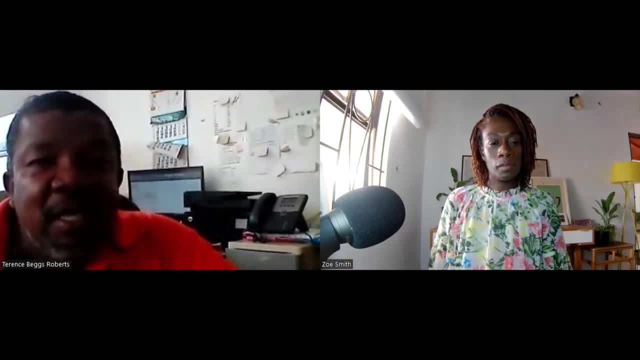 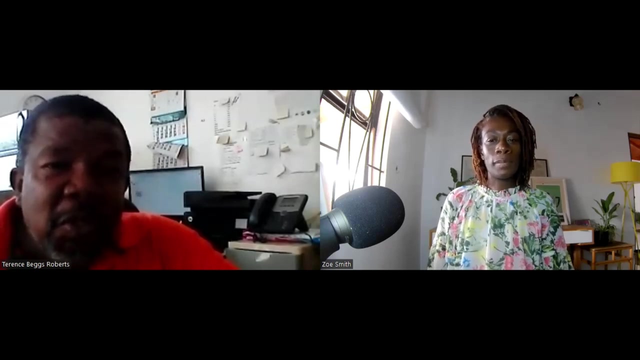 and so- and maybe it is the only company in Grenada that you can come between, let's say, 7 in the morning and 7 or 7.30 in the evening and find somebody here who is willing to listen and help, And that's one of the reputation that we keep and we are proud of that. we are not hell-bent or rigid in terms of like. in most cases some people 8 to 4.. 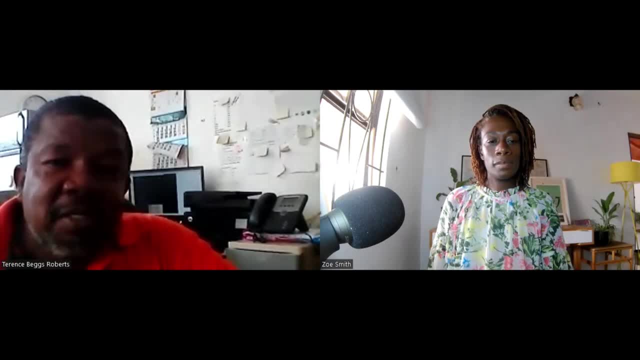 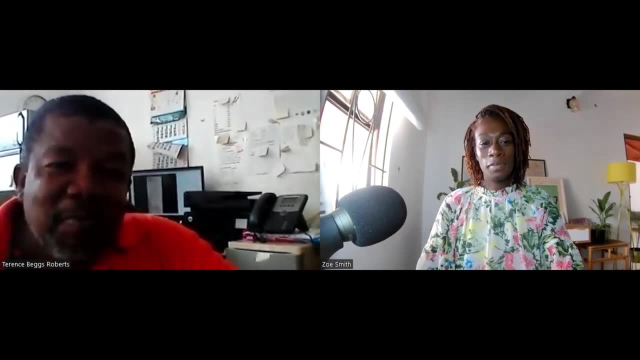 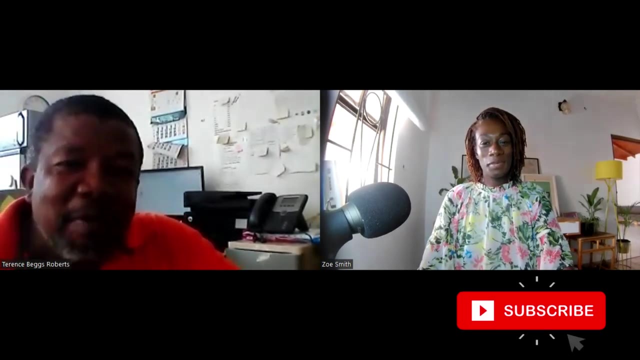 No, 4 o'clock is not B Caribbean closing time. You come 6 o'clock and you find B Caribbean. You come Sunday morning And you can find B Caribbean. You come Sunday afternoon to B Caribbean. You call B Caribbean 7 o'clock this evening and somebody will answer the phone. 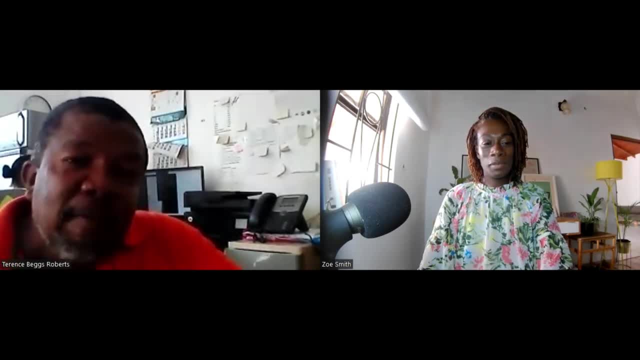 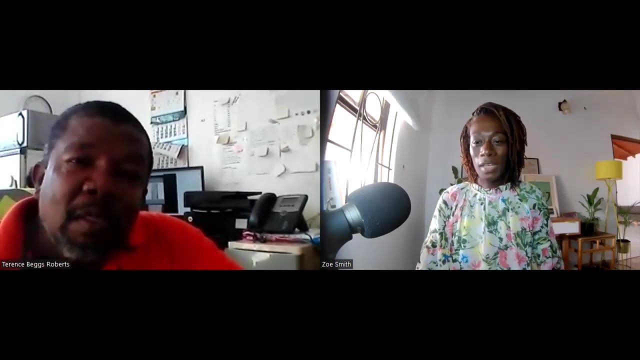 And will answer the phone in the most pleasant manner And will stay on the phone with you as long as it's necessary, Whether it goes to 7.30 or to 8 o'clock. So yeah, That's really good to know. 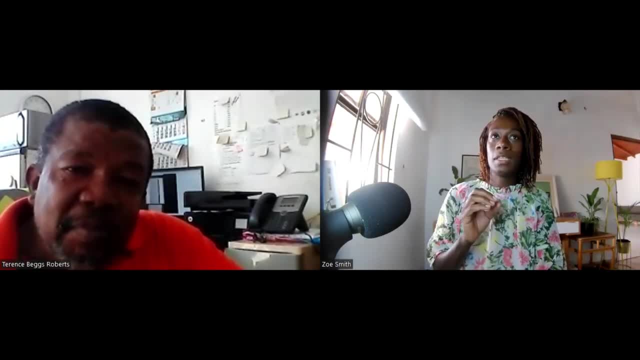 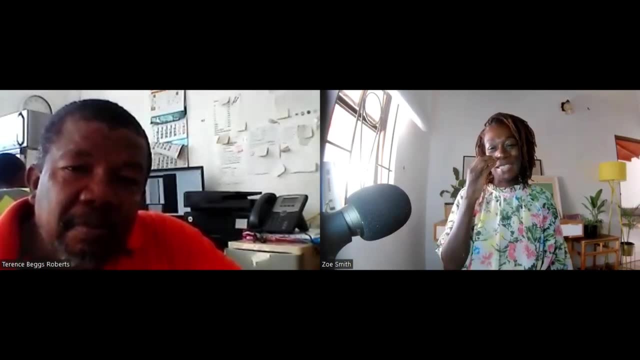 And I've already got some gems of wisdom from you already, because I didn't know that you had to clear within five days. I'm like, oh, it's at the port, I can pick it up whenever I want. I didn't realize that there are charges that rack up, which is why it's so important to work with a broker. 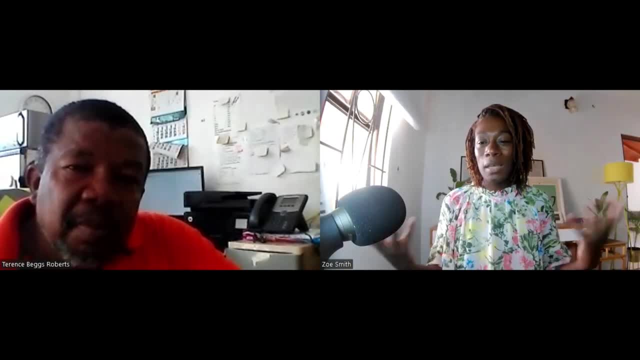 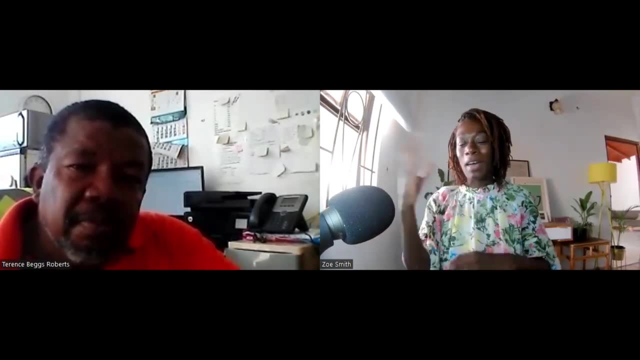 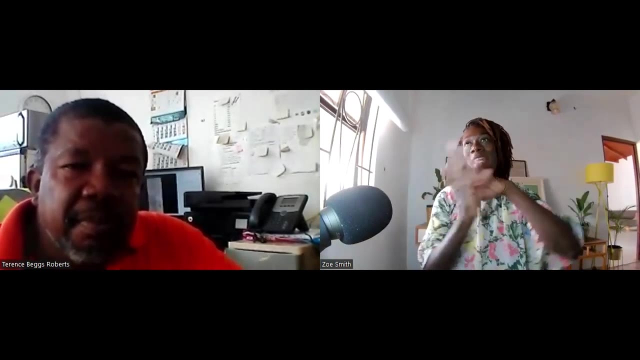 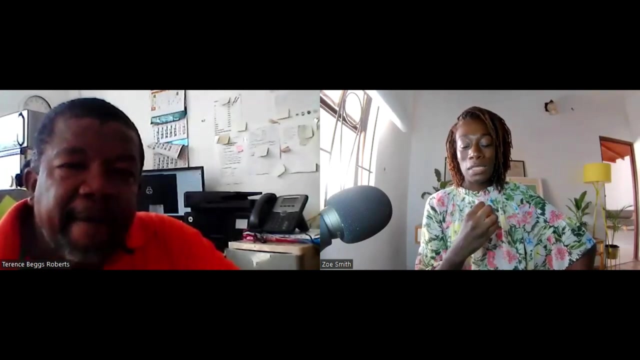 Because for those of us coming from the UK or the US, when it comes to ordering stuff or shipping stuff, it's so much more simple Because you have the Royal Mail, You have Amazon, You have. it's quite simple. But I think for when it comes to moving to the Caribbean to understand how to navigate all of the sort of different elements that come in with shipping items, it's really important to work with someone who understands the field fully. 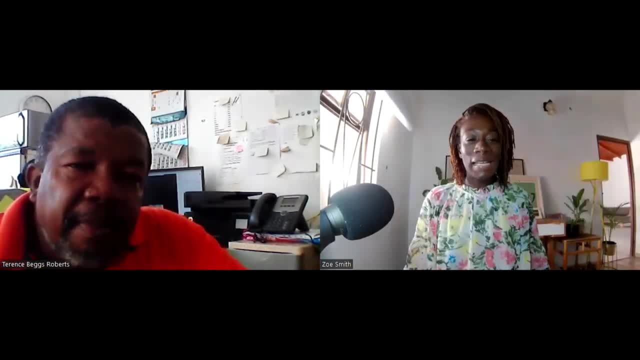 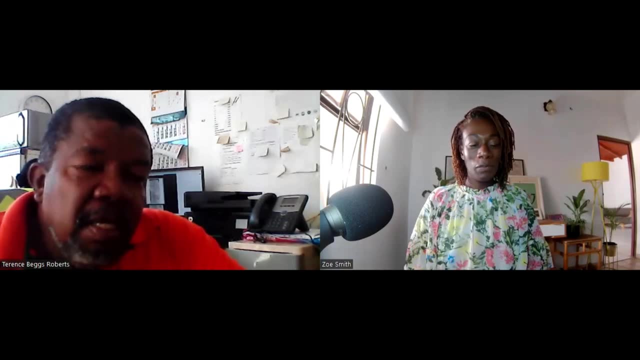 But let me take it back a little bit further. What exactly is a customer broker And what does a customer broker do? Why might people even need one? Okay, to clear many shipments. the ordinary person would not be able to assess the customs system. 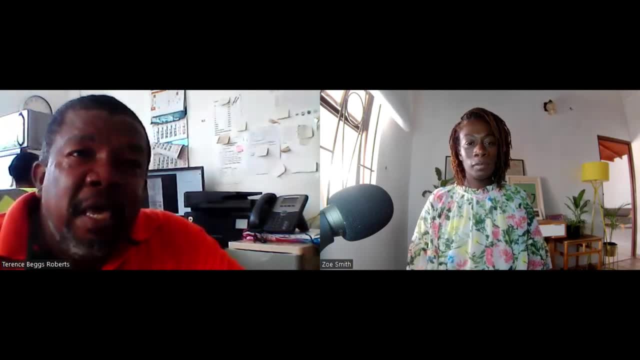 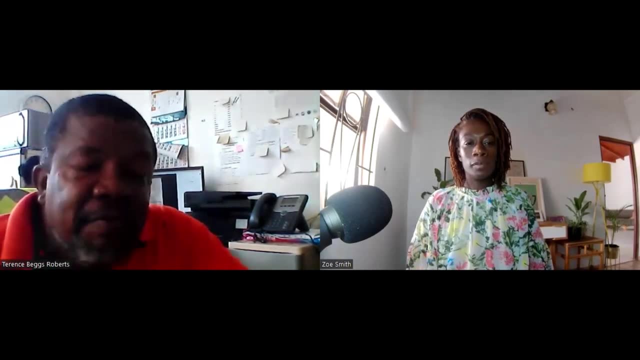 It's just like you need a certified lawyer to represent you in court, And even if somebody has to The skill and expertise but doesn't have the certificate, they would not be allowed to come in court to represent you. Something similar to that: a doctor needs that medical certificate to be able to practice medicine, to be able to assess the custom system and to prepare certain custom document. 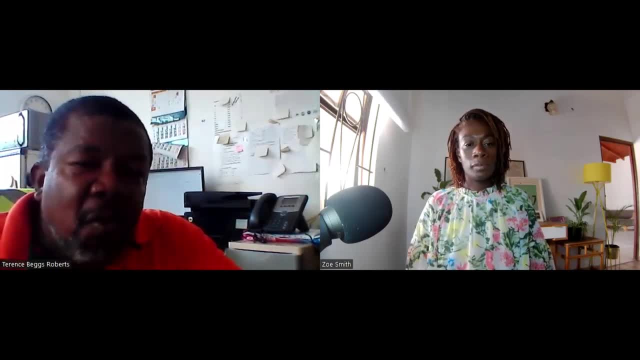 The customs Insists that only a certified broker would be able to get on to the system and to prepare that document that you need. So, for instance, if you have to make what ordinarily we will call an entry, But what customs would call a declaration, 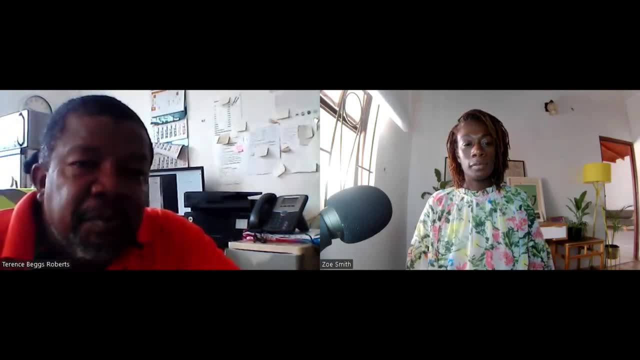 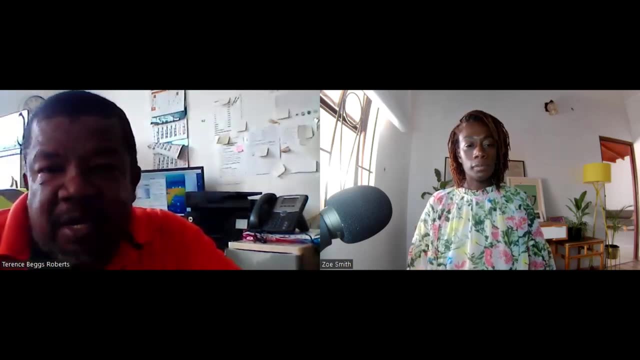 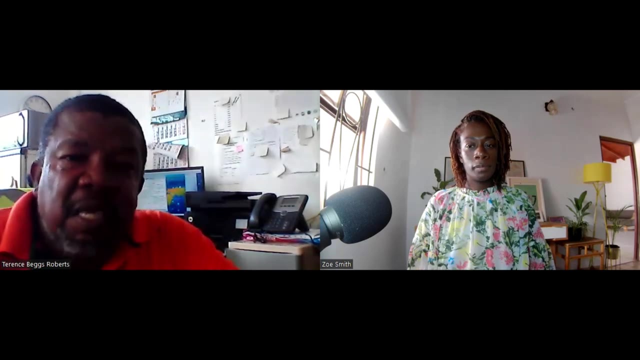 So that you can clear Your shipment. One has to be able to assess, Get onto the custom system To prepare that document. If you are not a recognized broker, You would not be able to get onto the system. It's not something that you can take a pen and paper and just write. 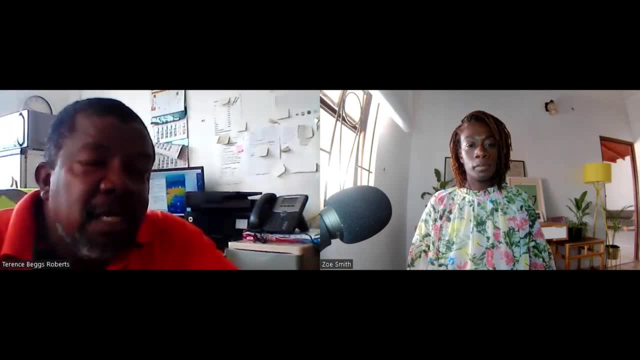 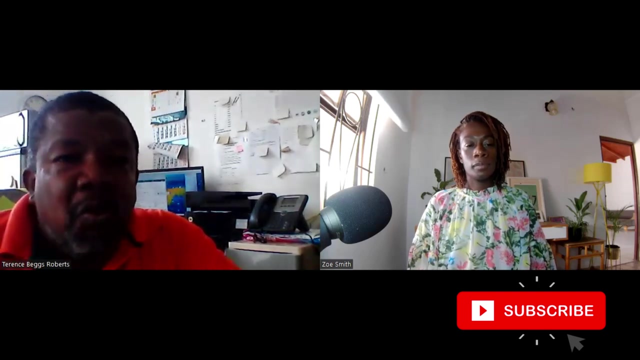 Okay, So the broker is one who is able, Which puts up What should be knowledgeable In terms of what you, as a An importer or an as an exporter, needs to have. The broker needs to know the rules concerning importation and or exploitation of goods, because there are certain goods. 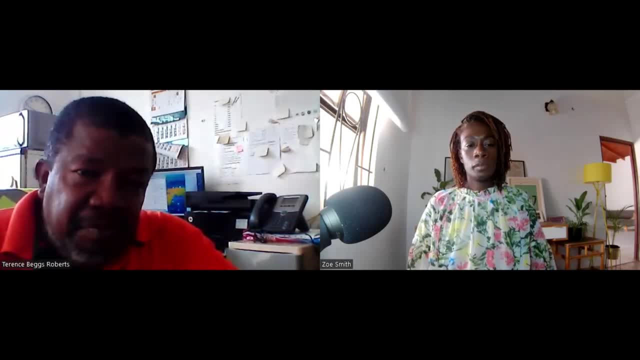 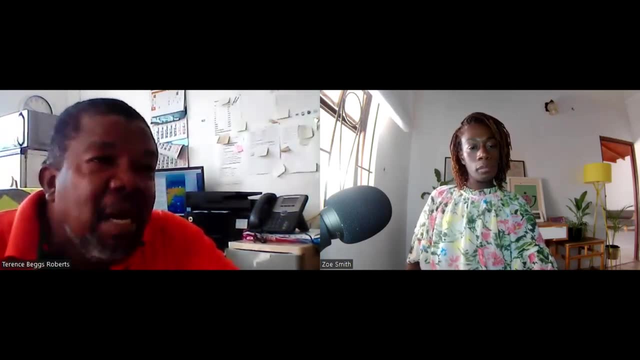 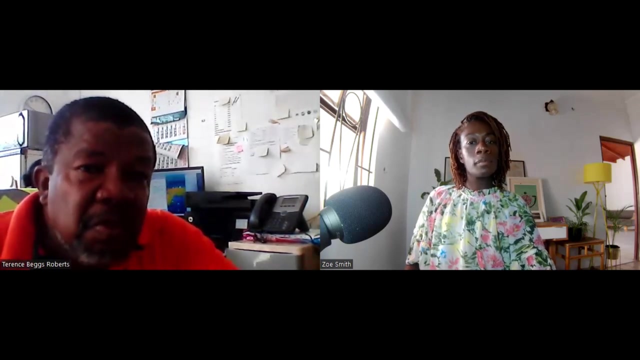 That require additional Work. For instance, if you brought in A simple item like clothing As nothing that you need specifically, But let's say you want to bring in something like A plant. It's a yam, A piece of dashing or something like that. 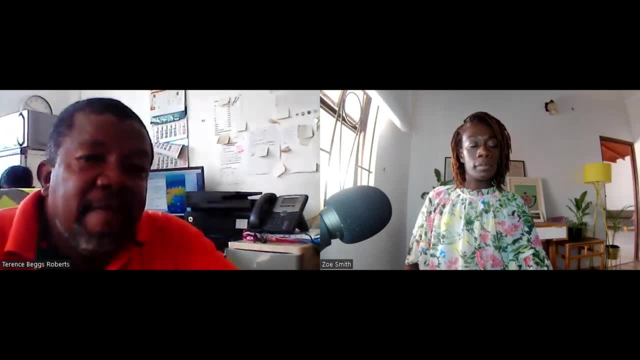 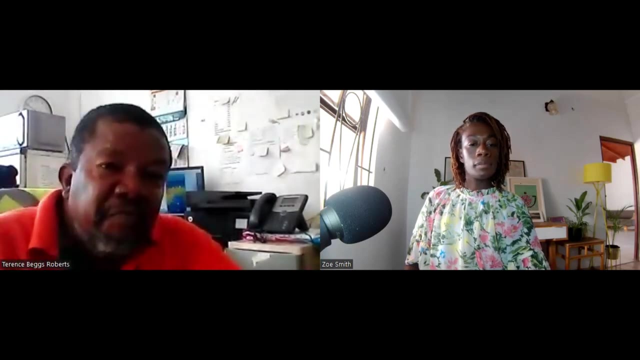 Then that pizza, yam dashing. Would not you not be able to clear that yam dashing, Unless, let's say, in our case, You have to go to the agriculture department, Provide them with information, Prepare the document, But all of that document to do that? 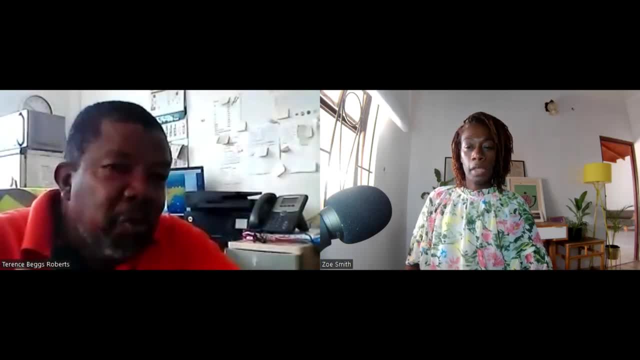 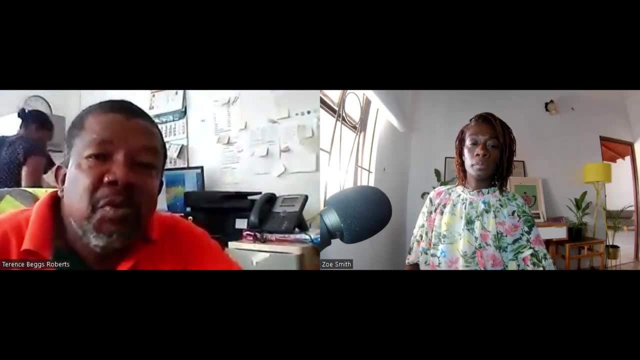 Is done On the same custom system, So you, as a member of the general public, Would not be able To go onto the system To prepare that document. The broker Has to know That what he needs to do So he can just eat. 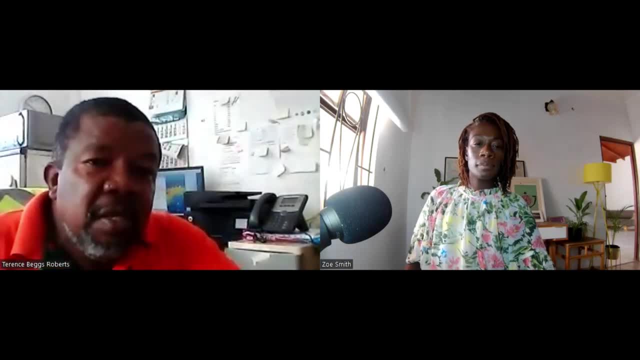 Take you to the port to clear your dashing or yam, Simply show up. No, That wouldn't happen. There are certain goods that require License for different reasons, And the broker Has to know What goods require license, How to apply for the license. 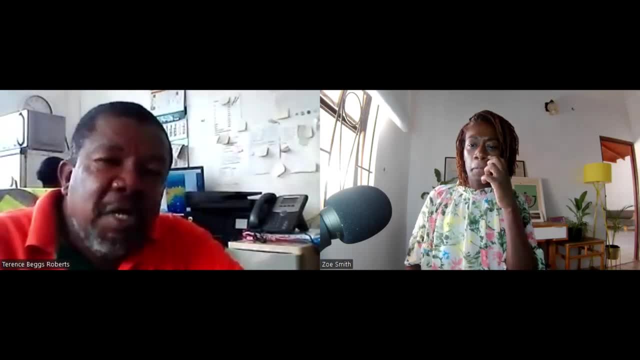 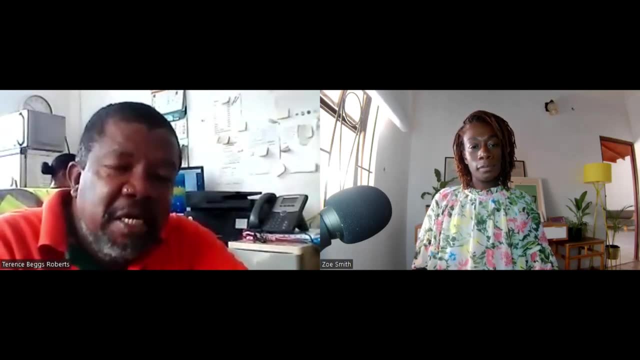 And such a like. The broker also has to be familiar With, let's say- and I know this is one of your be concerned- The returning nationals What they are entitled to? Okay, Unfortunately, many do not understand what is available to the returning national. 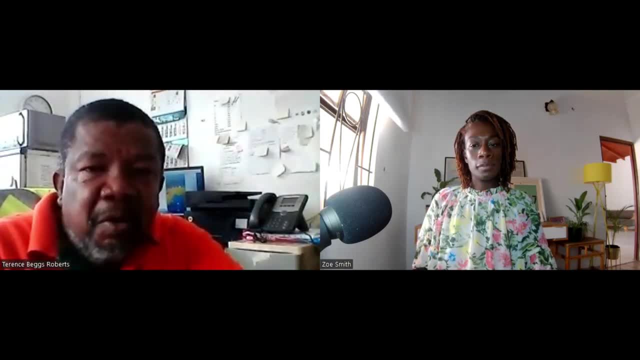 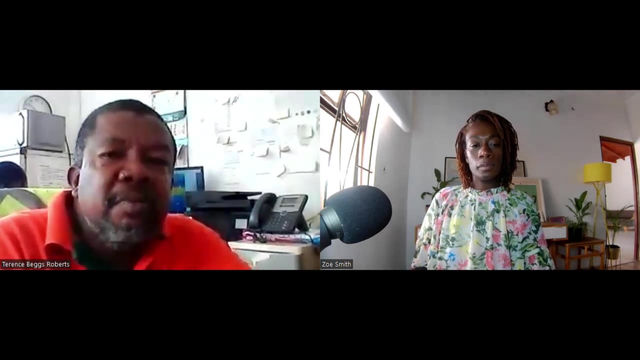 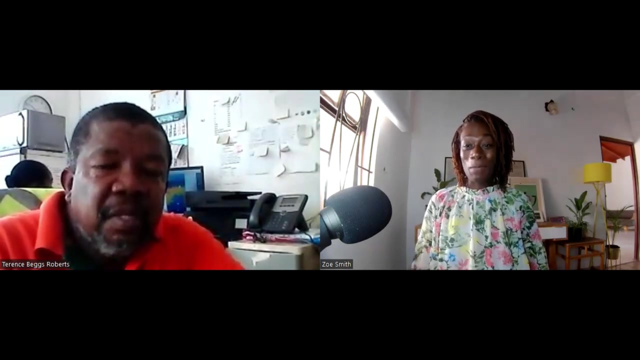 What is available And some persons who should not be paying some monies to customs end up paying monies to customs simply because of lack of knowledge on the part of them and on the part of the broker that they might have. Okay, And we definitely want to go into the returning national's details as part of this. 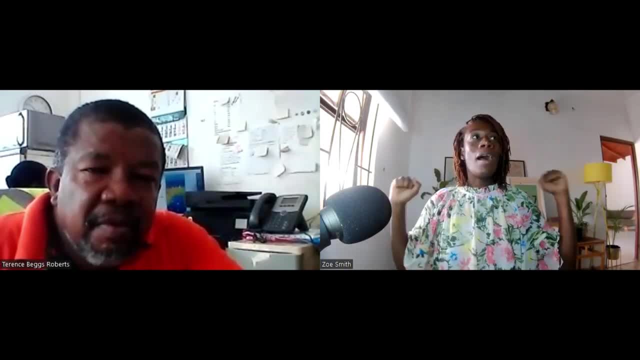 But one of the things that I really want to know is: say I'm in the UK, I'm ready to move to Grenada, or I'm moving to Grenada in six months' time, At what point do I need to Do? I need to engage someone like you. 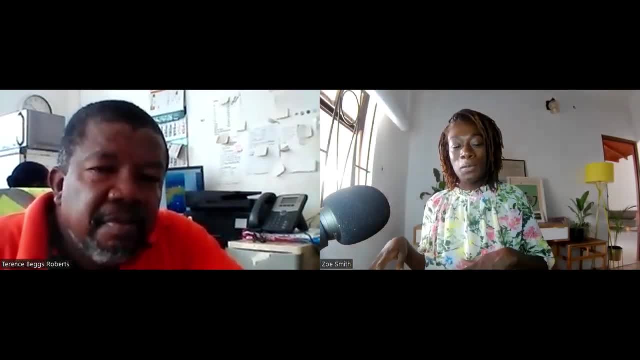 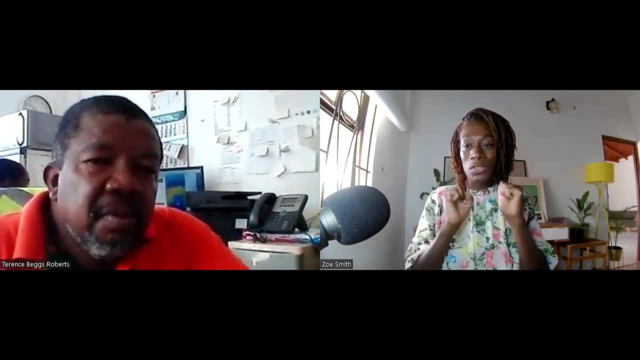 And at what levels? If I'm shipping a barrel, do I need a customs broker? If I'm shipping a container, when do I need it? Does everyone need a customs broker? Every individual need a customs broker, And at what point do you decide if and when you need one? 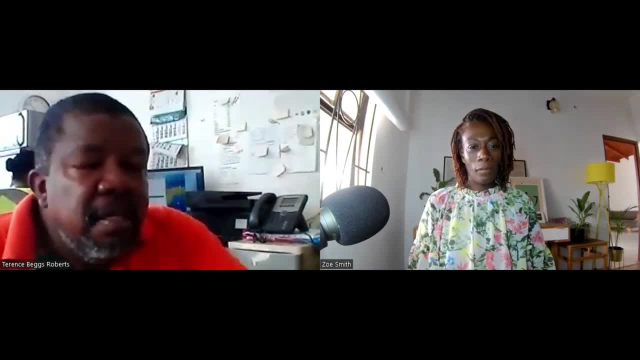 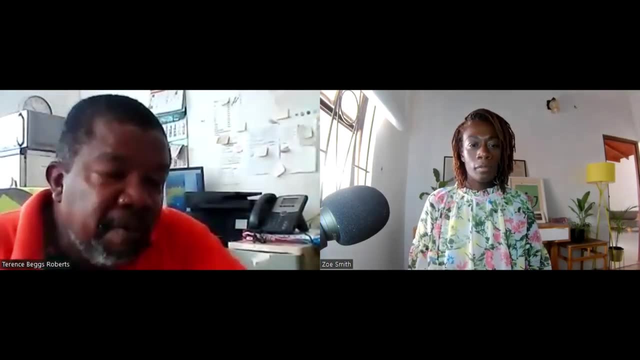 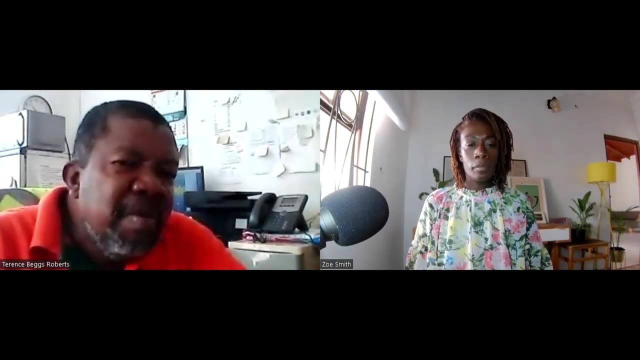 No. The answer to that is probably no and yes, I would think that you need to engage a customs broker, because Prior to any shipment, so that you fully understand. it doesn't mean that you would need him to clear that shipment, But at least you would know what to do and how to do. 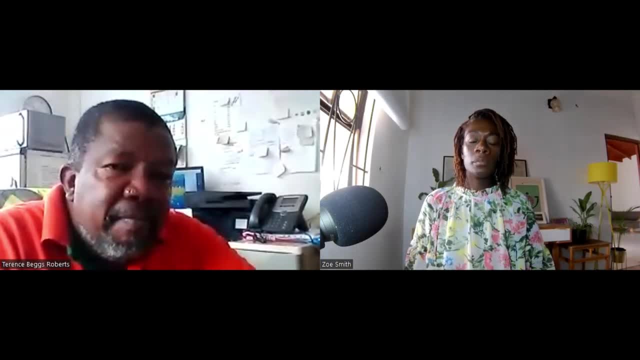 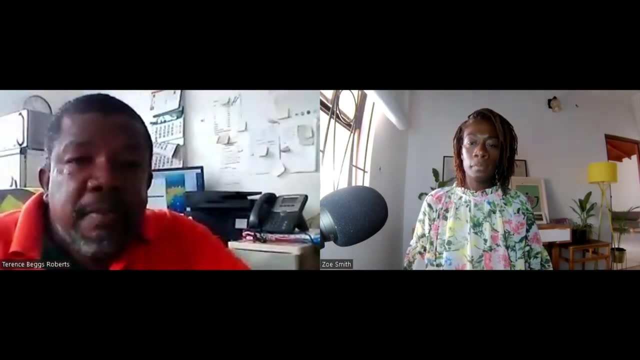 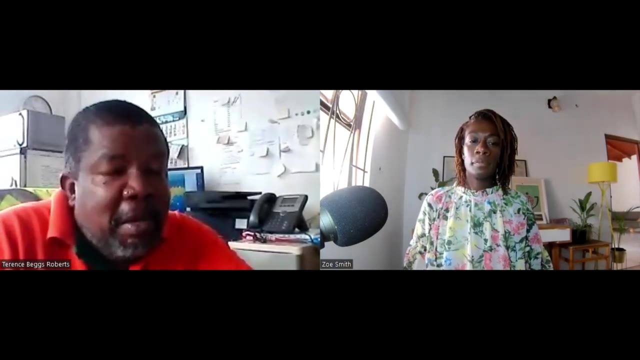 For instance, you might ship a simple barrel. Now what's a barrel? A barrel doesn't say anything of the content. A barrel is simply what you're going to put goods in. Normally, when we see a barrel, we think foodstuff. 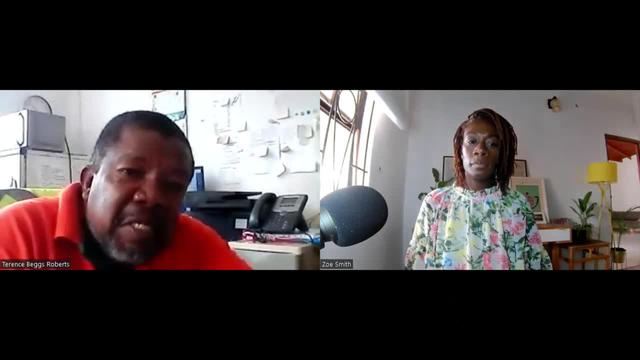 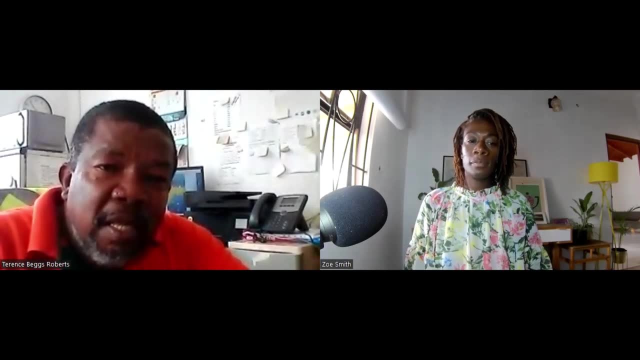 probably a bit of clothing, maybe a smaller plant or two, But a barrel could have anything in it. A barrel could have commercial stuff. Now, if you send What we would ordinarily call an ordinary barrel, For simplicity we say an ordinary barrel. 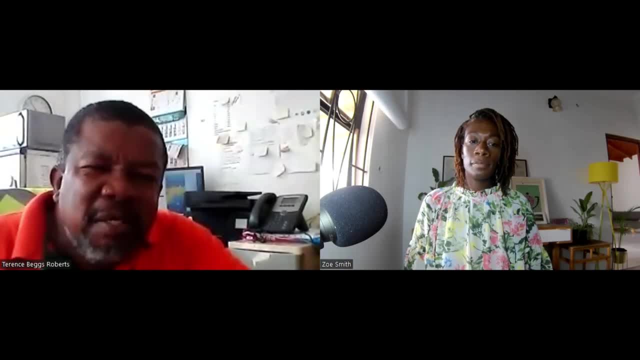 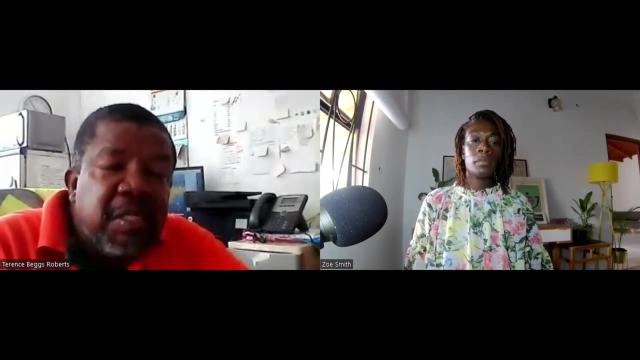 Basically some foodstuff, a little clothing, nothing to talk about. That doesn't require a customs broker at all. You can come collect the document at B Caribbean, pay B Caribbean a small fee that we charge, go over to the port and clear your balance. 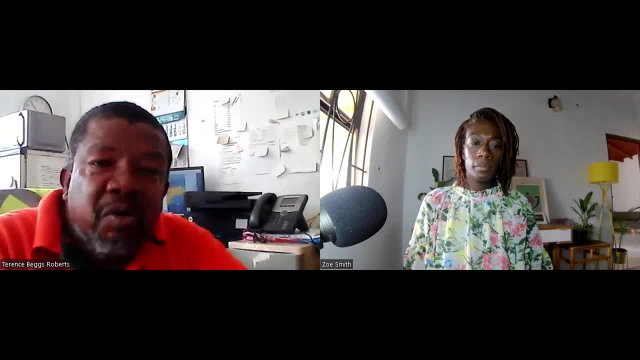 And if it's not busy, within 20 minutes, half an hour, you're in and out of the port. Okay, But suppose that barrel upon examination customs. realize all you have there is clothes and there's things to sell. It's the same barrel. 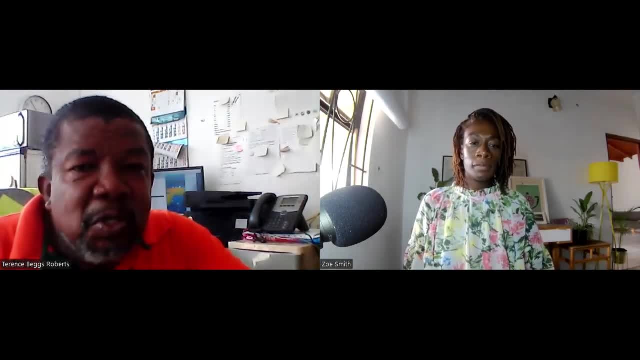 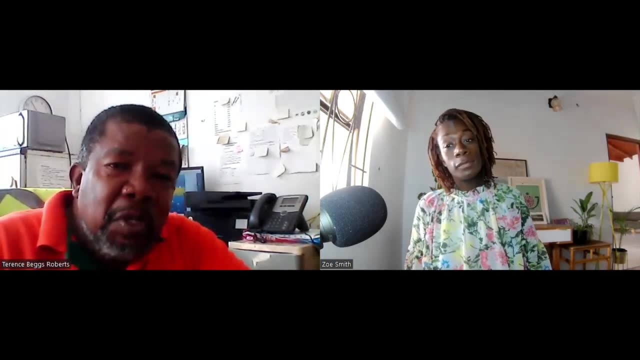 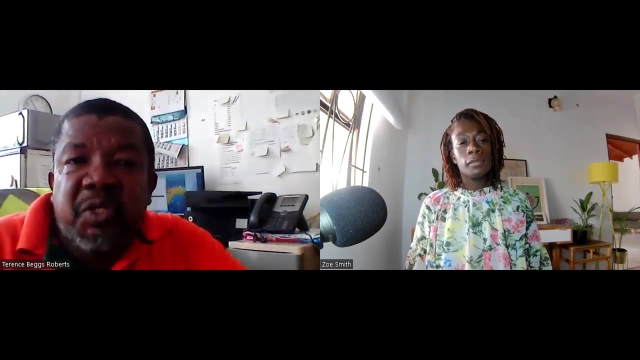 And that's a whole different matter. Now you're talking, they would say it's commercial, You need a broker. Okay, They will ask you for your invoices and things like that. They will want to get a document that shows how much you pay to ship. 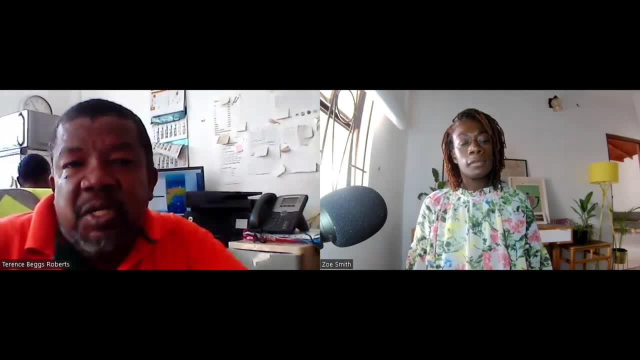 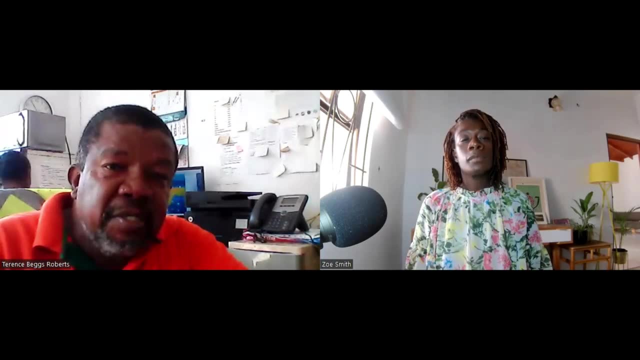 because they know, in Grenada the duties are charged on the CIF cost, insurance and freight. So the cost of the items added to the insurance, if it's insured, added to the freight, which is the cost of shipping. Okay, Okay. 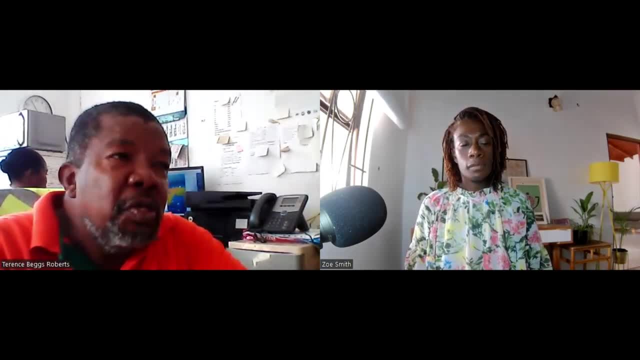 Now let's assume that you had a barrel of that nature. but you had not, you had never talked to a customs broker, So you didn't know. you thought to: the barrel is here, you can just go to the port, and then you find that you stopped. 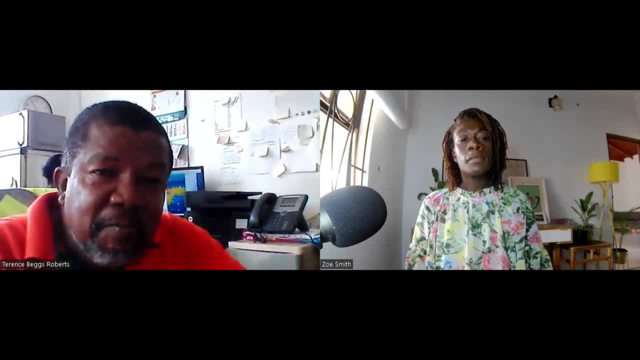 So now you have to go and try to get invoices, try to get the shipping costs and everything, And you would find very often, because, remember, we have five days, five days, and because you are not prepared for that, sometimes it takes you a lot more than five days to be able to get what is needed. 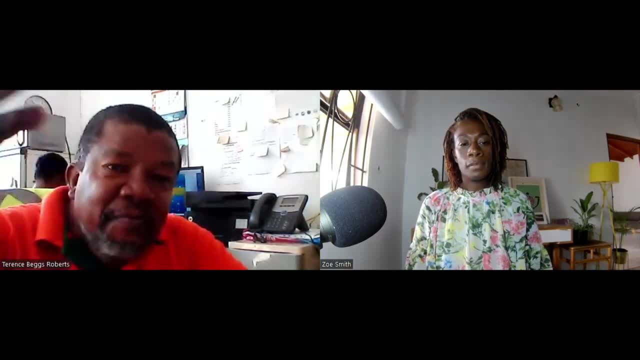 If you are engaging a customs broker from before you ship and you said to broker Beggs: well, I have a barrel of clothes coming down, it's for sale. Beggs can tell you: well, make sure you have your invoices, make sure you have the cost of shipping and such a like. 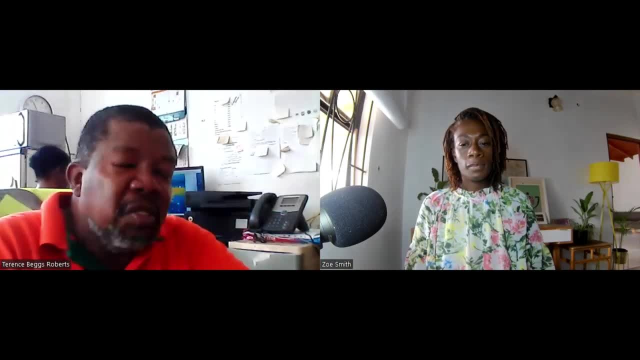 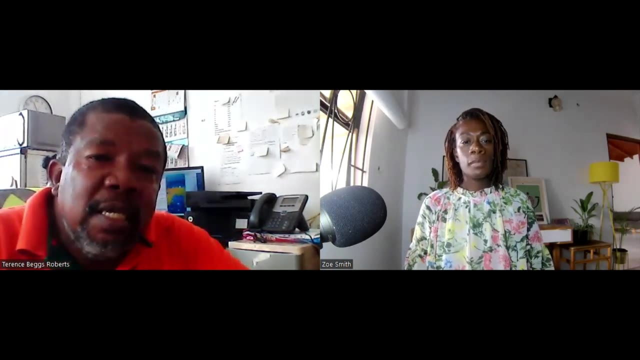 So when you come, everybody knows. So we go to the port and you have your invoices already. You have, as a matter of fact, if you have all the invoices and everything that is needed, the broker can prepare that document before you even go set foot on the port. 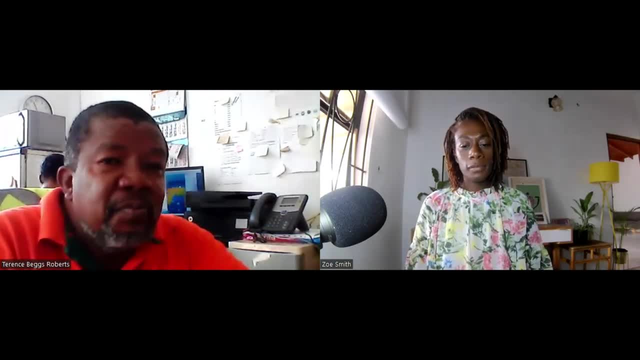 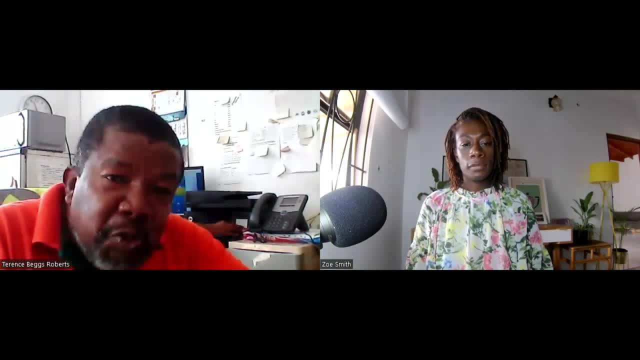 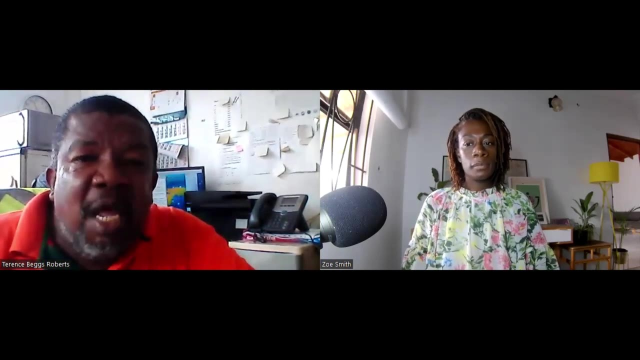 Even before the goods are arrived, the document can be prepared, the duties could be paid, everything. So when the goods come, you go over to the port and the customs would reserve the right to examine the goods or not. So sometimes they don't even ask to examine the goods. 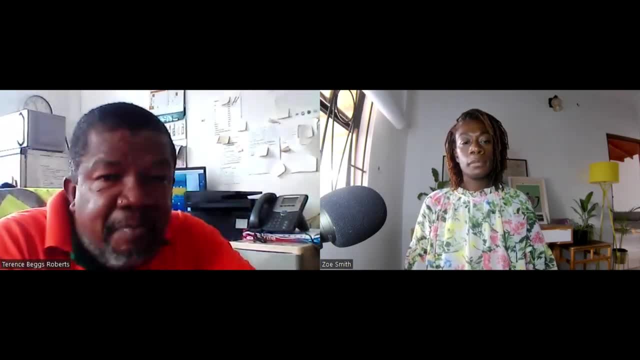 The duties are paid, the documents are presented to customs. they are happy with the document, they release the goods, you go to the shell. you don't even have to open the packet sometimes and you collect your package and you go. So that's what I'm saying. a broker should be engaged. 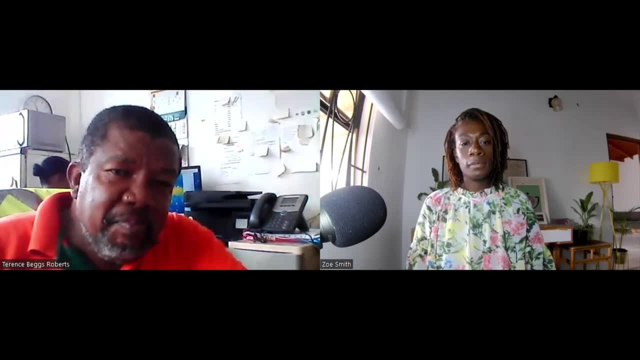 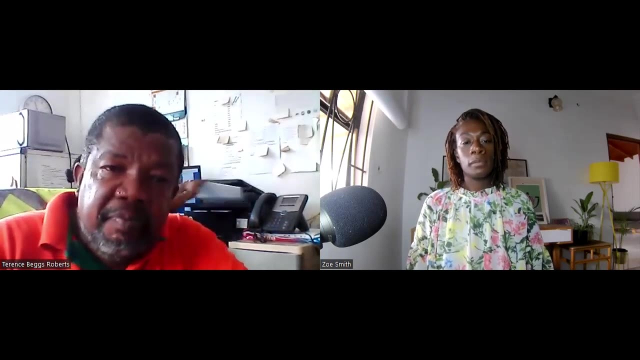 You don't want. for instance, even if you have a barrel and then you have certain items in the barrel that might be on a negative list or certain items that might require view of standard work or the Ministry of Agriculture. if you engage a broker very early and you say I have this in my barrel, the broker can say to you 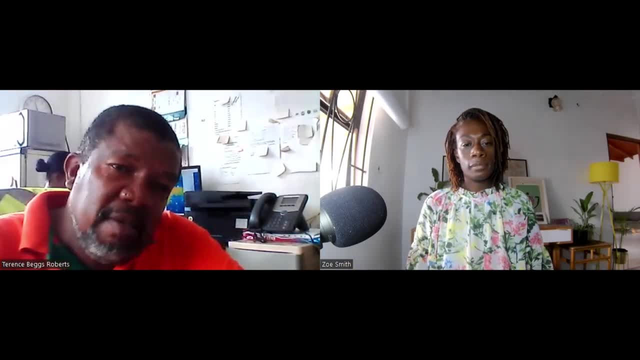 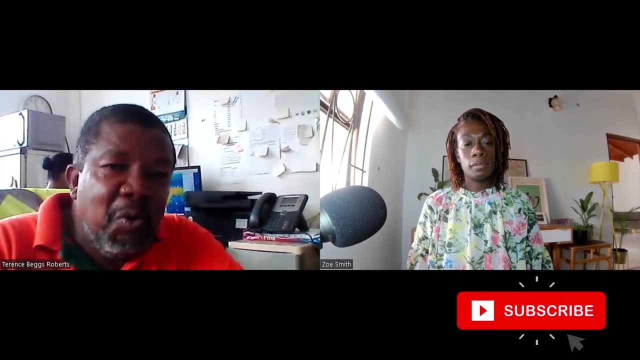 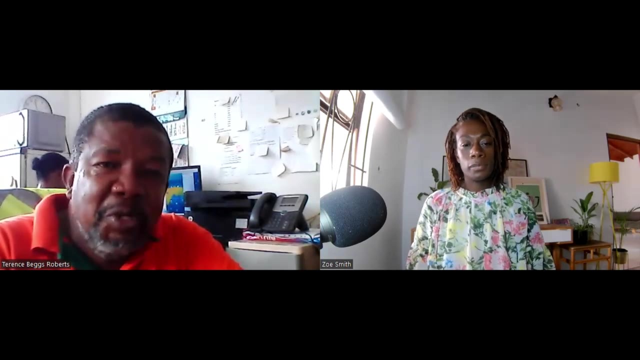 well you know, make sure you have to get this done prior to going to the port, and so you can save a lot of time and remember, like I said, you always remember- that after five, three days, the port is going to charge you rent, regardless of the reason for the delay. 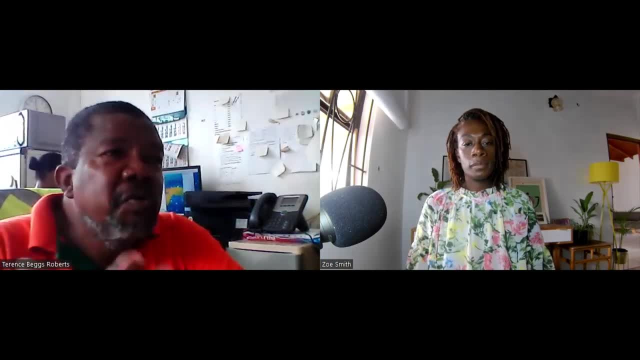 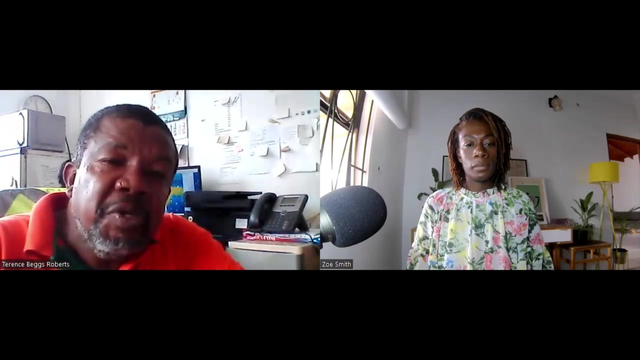 Okay, so the broker can be used as an advisor even before you ship. So you call the broker and he says: and the broker can tell you: okay, what you have there is fine, there is no problem. Even before you ship, the broker can give you an idea of what your duties to the government would. 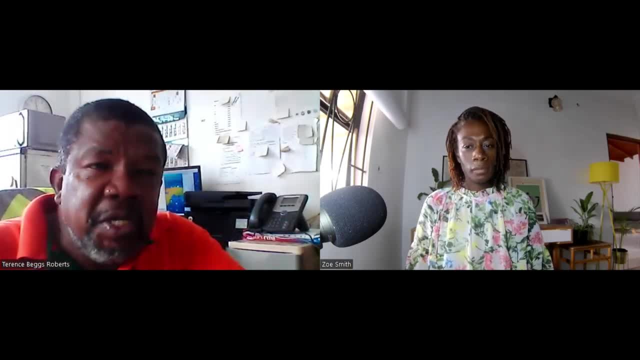 be. So you say to the broker: well, I have such and such, And before I go further here, I can tell you outside there, for some strange reason, there seems to be a lot of misinformation, And the sad thing is that very often 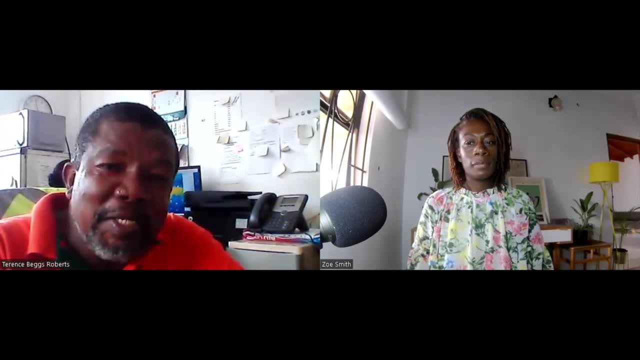 the brokers have to give the correct information at a time when it's a bit on the lead side. So you still have persons bringing vehicles five, six, seven, eight, nine, ten years old and expect to get concession on them, Because some of them are misinformed outside. 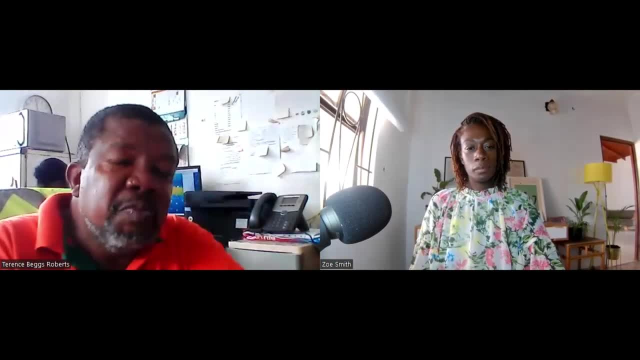 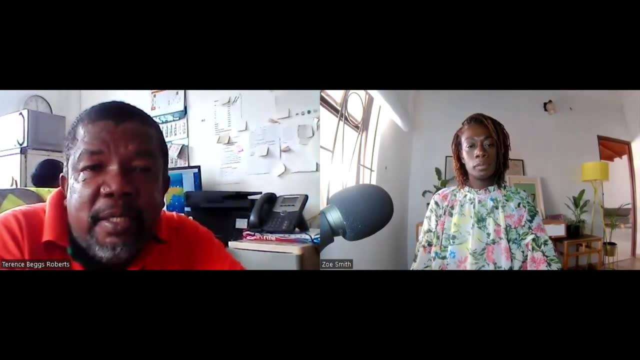 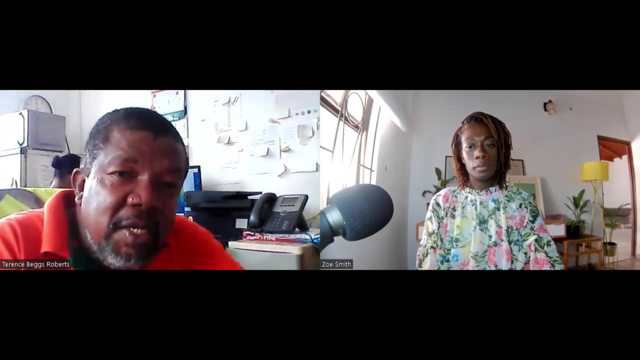 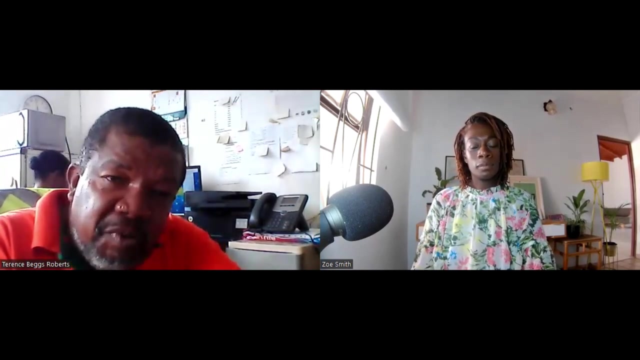 And the ten years that are spoken about has nothing to do with concession. so persons bringing their vehicles and vehicles five years and they might be a returning national and they expect to get concession and then they are told: sorry, no concession is given to on vehicles above four. 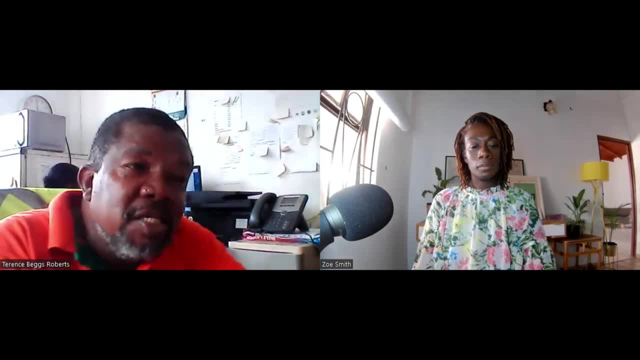 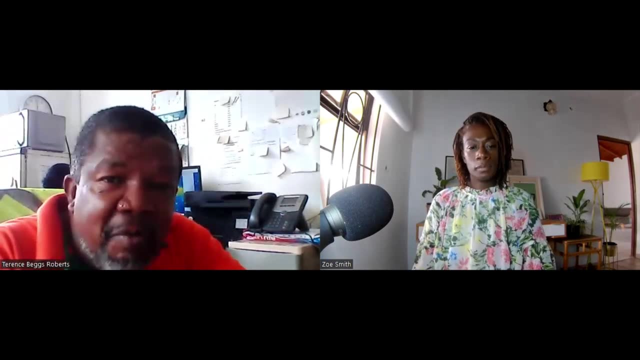 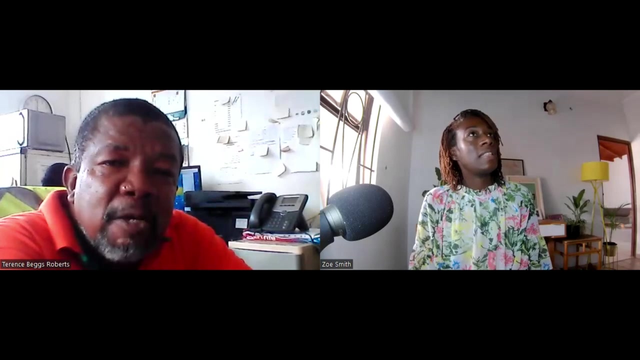 years old and instead of getting a concession where you should be paying maybe thirty or forty thousand dollars to clear, there is no concession, you have to pay seventy or eighty thousand and you know so. the broker is absolutely necessary, right? okay, even, just advise me here. yeah, and I think that's one of the things that feels overwhelming to people when they 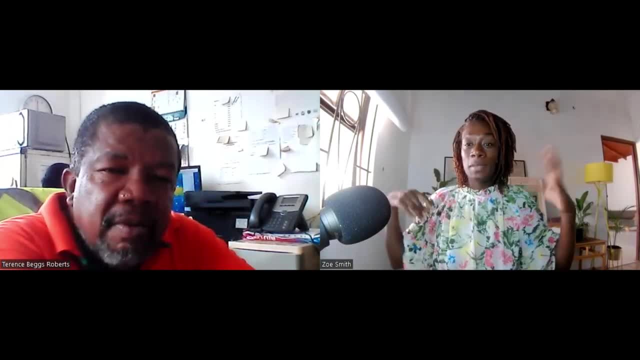 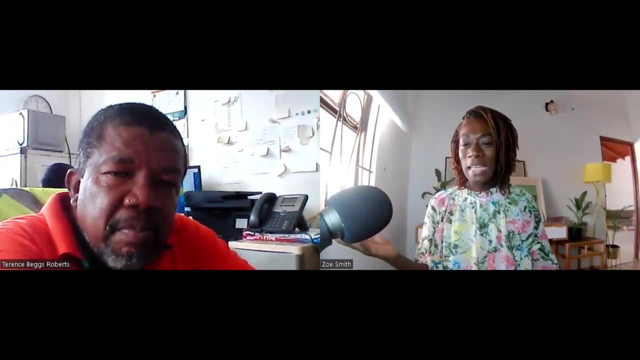 think about shipping, whether it's from the UK or the Arab world, us, it seems to be that uncertainty. it's like: how will this be classified? what will this be valued at, even when it comes to second hand or used items? um, it's i, as someone who's been to the 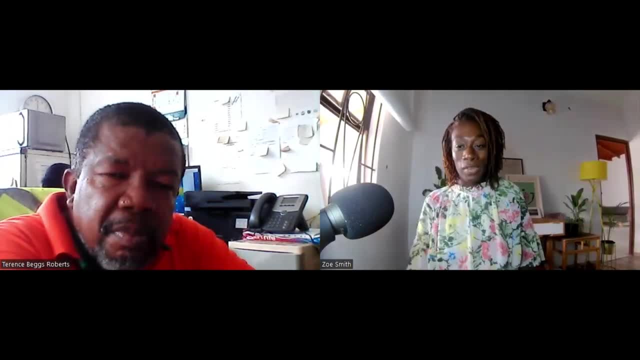 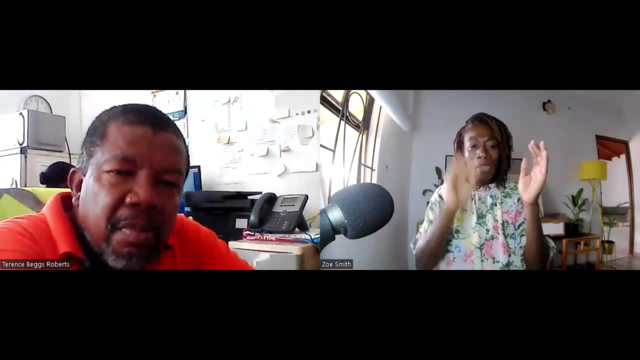 port myself. it's a sort of you never know what the final figure is going to be, and it shouldn't really be that way, because there is a catalog, whatever a book that you can refer to that has all the facts and figures, but i guess, coming to a broker beforehand explaining exactly what you have, 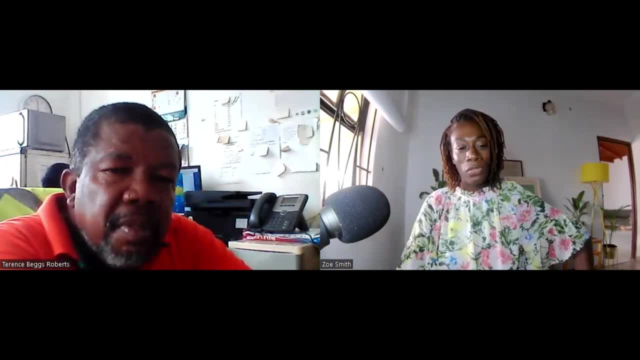 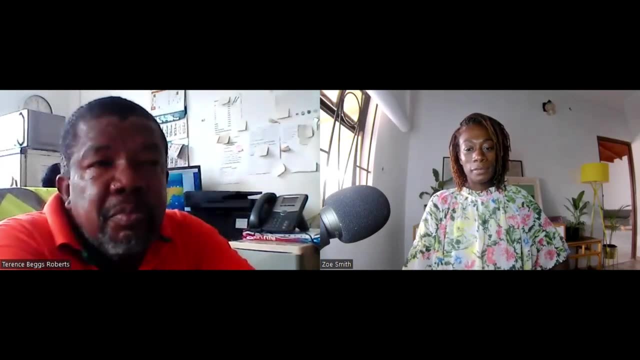 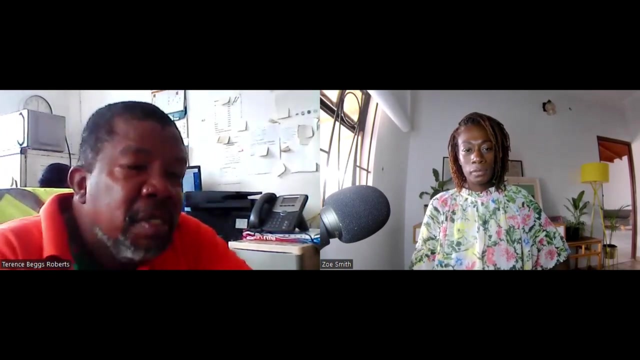 it reduces that like, uh, how much am i going to be hit with sort of feeling: yeah, one of the years ago, years ago, that was something that they sort of worked with. today is different, and i tell you why. in the early days where custom valuation was done by under what was called the brussels arrangement, 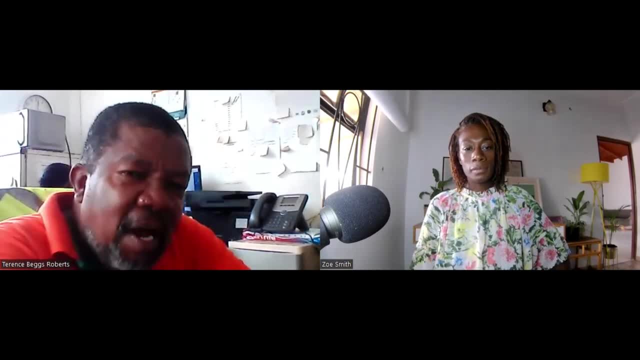 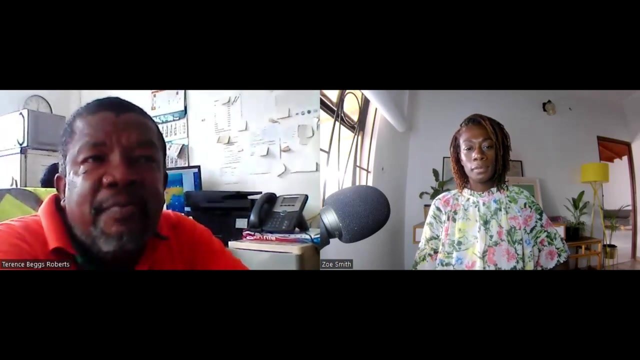 where market value values were used to determine the value of an item. but the w trade organization has since recognized that the market value system is unfair. it's unfair to the person who, to their skill- skill of negotiation- can get a better value and therefore bid in bank and other barriers around their value. you should not be punished because of 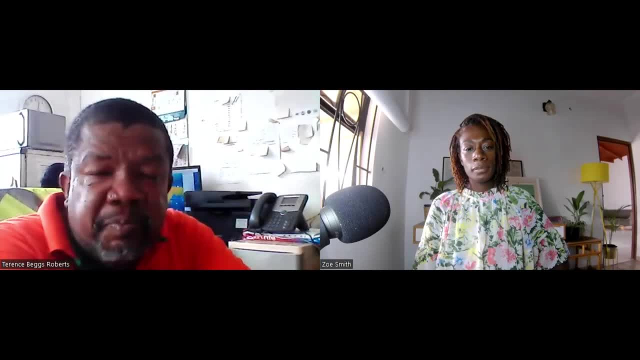 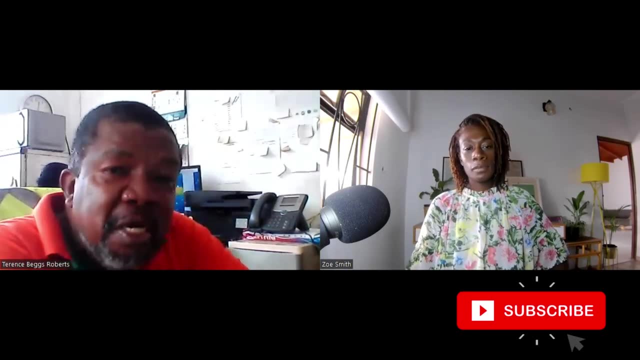 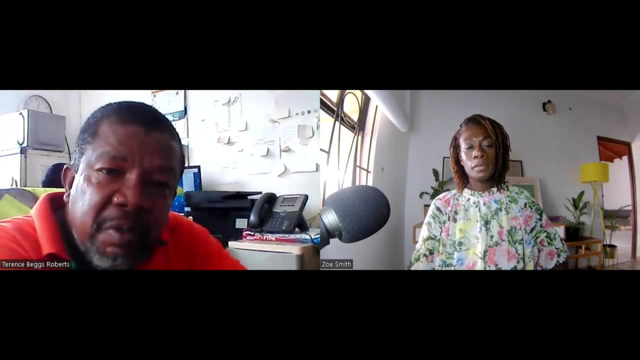 their that skill. so i went, walked into a store and i got a fridge for five thousand dollars. and you walk in and you were a very good negotiator and you get the fridge for four thousand dollars. you shouldn't be punished because you are a good, you know- negotiator. so what the wt has since. 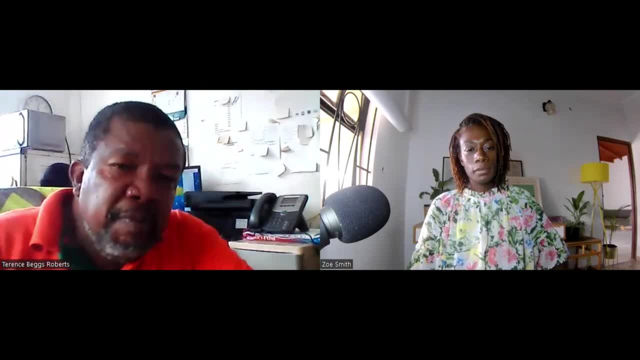 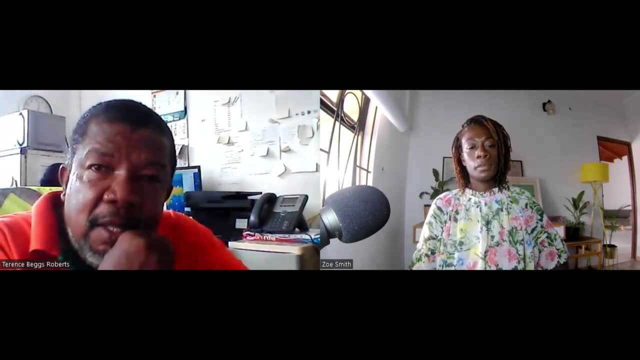 decided that valuation would be done from the bank toUSE, and that choice was that the much greater that value is made was about that so, and so they started investigating that trade. so the hartford institute done on the price paid or payable. So once you can establish that this is the price that you 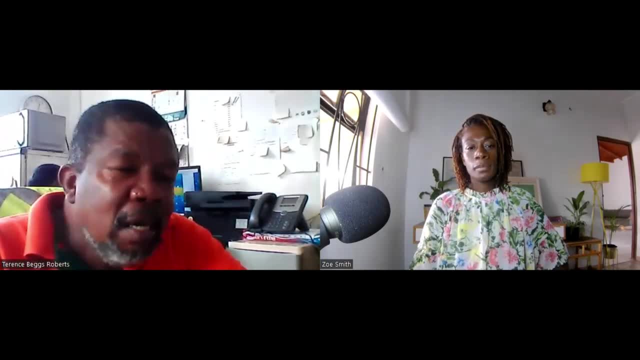 pay or have to pay. customs really have no choice but to accept that price. However, many persons do not know that That's where partly the broker should come in. Also, customs reserve the right to ask one to be able to kind of prove that's what you really paid. 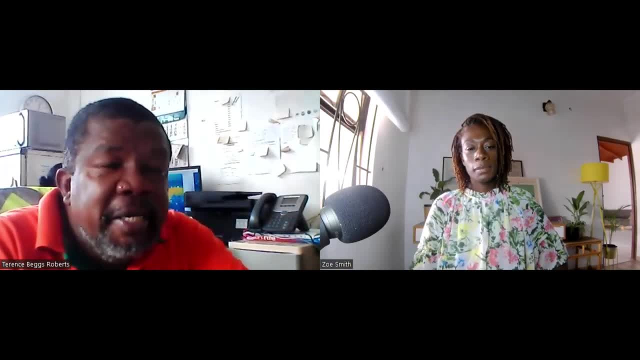 Again, if you touch a broker early enough and you said to the broker: well, I want to bring in such and such, the broker can ask you or advise you to pay for it in a manner that provides some kind of evidence. So there's certain things like maybe a credit card bank wire. 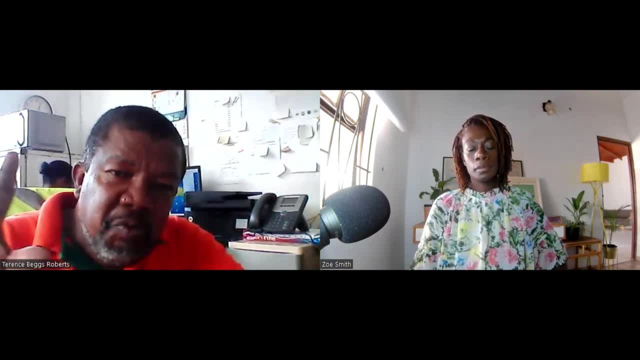 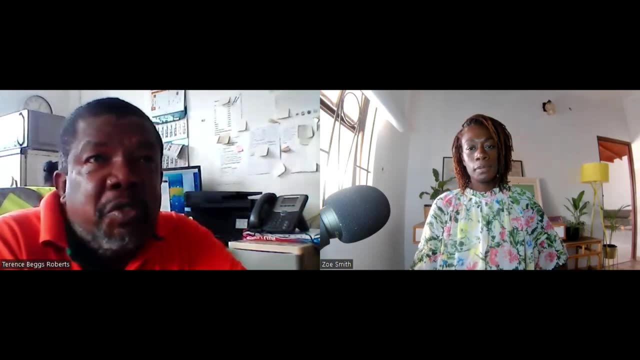 that you have a piece of paper that says you did pay this for this, some things like that. Rather than OK, you just walk in and see what I paid. that, or else I paid it, And strangely, I paid it with cash. 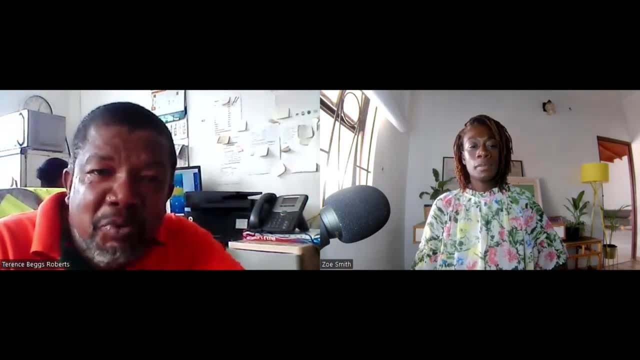 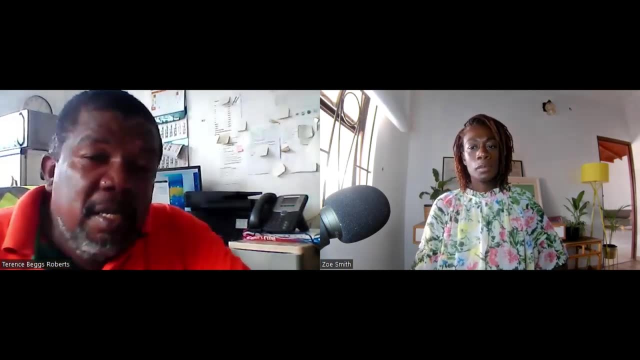 because customs always say that you cannot prove that you paid something. you paid that amount in cash, even if you have a receipt. What they say is that you could ask the person to write your receipt for any amount You could pay- up to 10,000, and you tell them write a receipt. 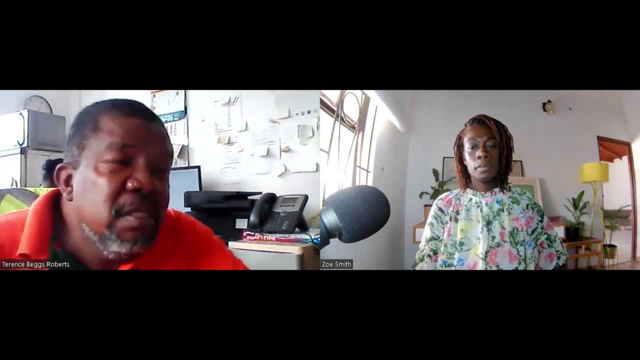 for pride. So we would advise persons Based on the item, particularly something like a vehicle, because the average duty on a vehicle, a used vehicle, is like 160, 160% of the cost, insurance and freight value. So 160% if you get a red deal you. 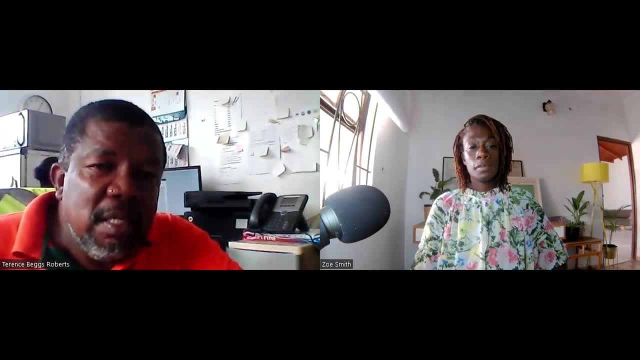 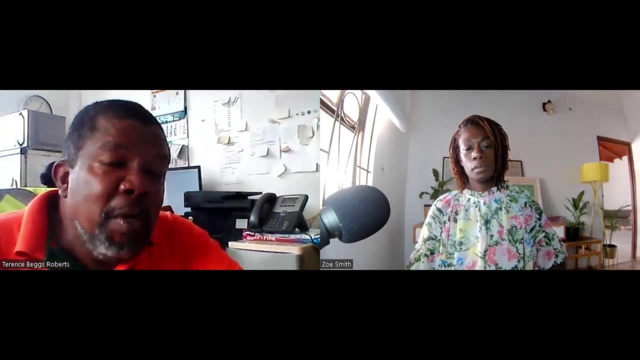 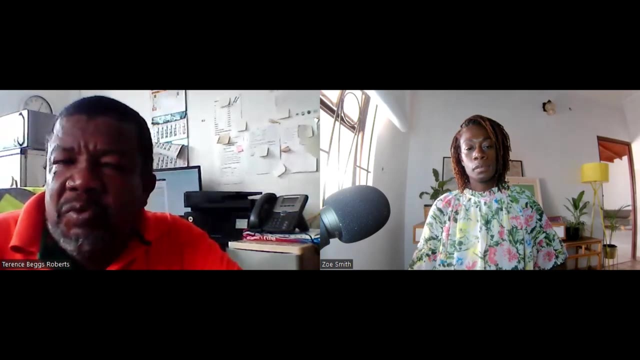 want to make sure that customs accept that deal, And so you want this. You want this. You want to bring in something that will establish to customs that that's exactly what you paid, And the truth is, once you can prove what you paid for it. 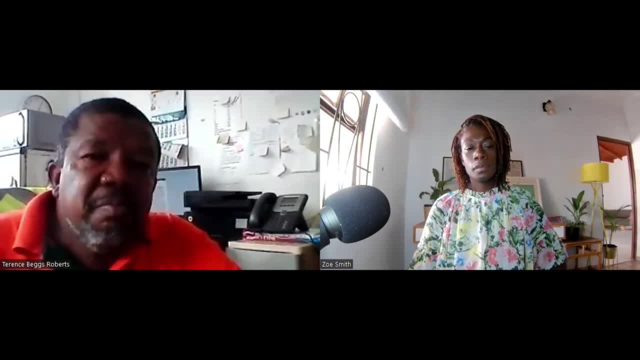 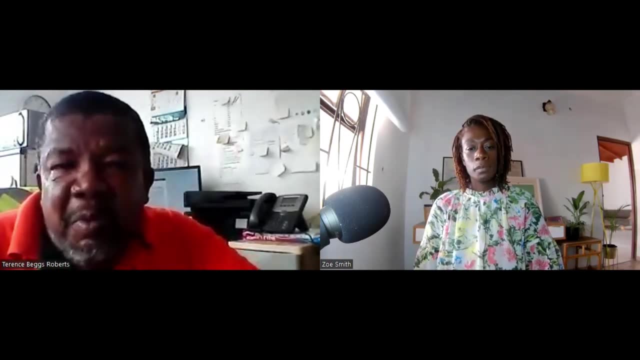 customs really have no choice but to work with it And again change where you have the broker, because customs sometimes will want to argue: no, That's not what you paid for it, That is, you know that price is too low. 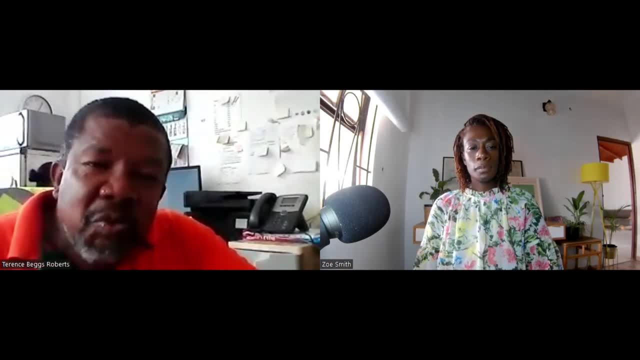 That price is too low. No, No price is too low, No price is too high. If that's what you pay, that's what you pay. And if you are a good broker, a good broker will see to customs My client what they paid. my client is not going to pay a cent more.